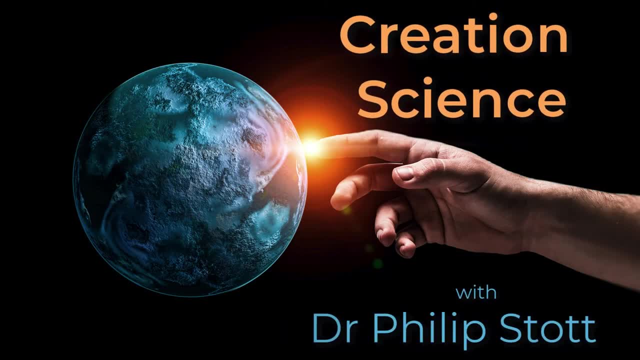 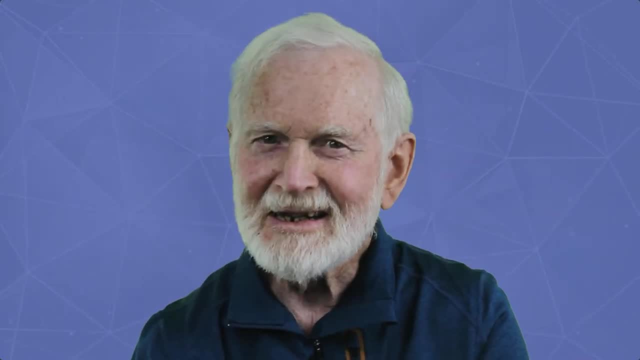 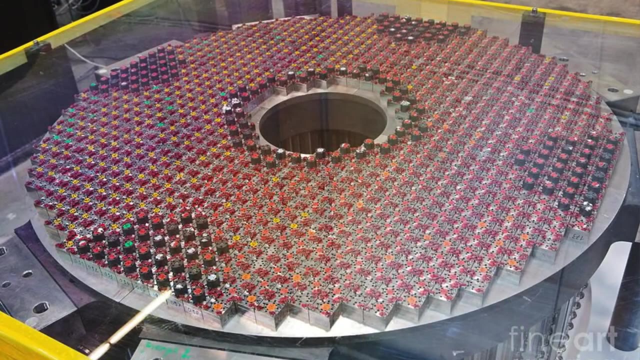 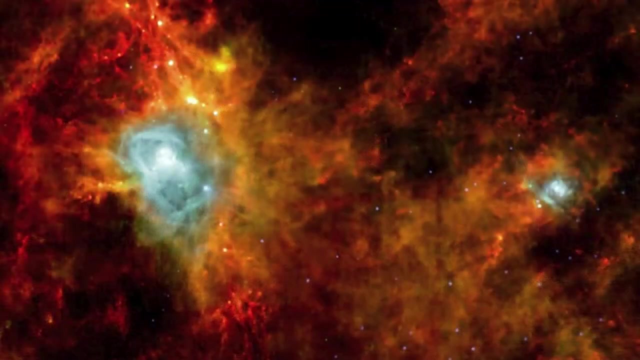 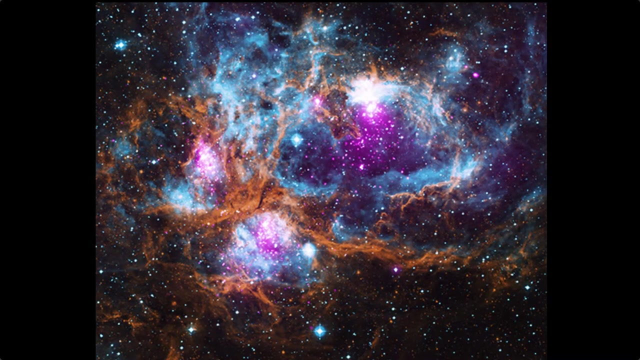 Brilliant engineering and technology have produced telescopes with astounding light gathering power. They can deliver amazing pictures of what are usually referred to as astronomical objects. These pictures are nothing like what an observer would see by actually looking through a telescope. When I visited the very large telescope at Sutherland a few years, 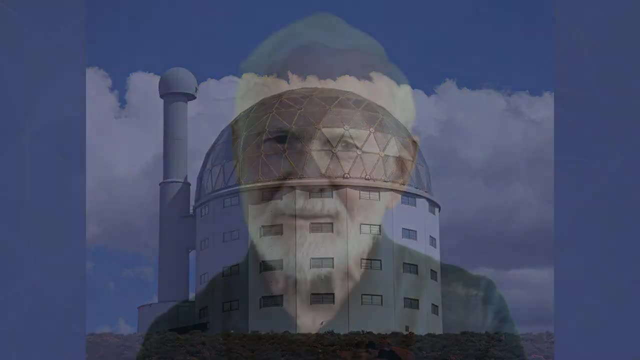 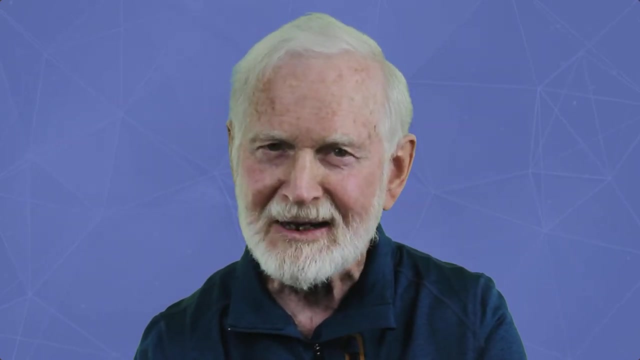 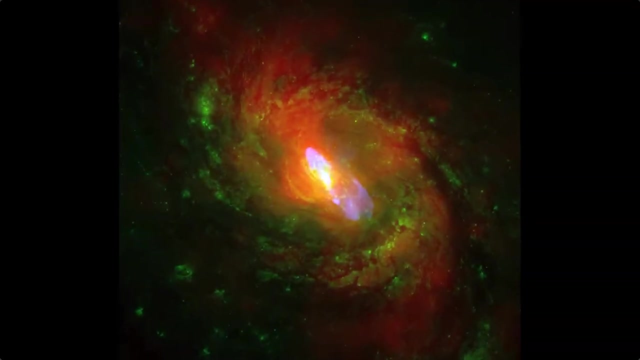 ago, I asked if any photographs had been taken with it. I was told that the staff didn't have the time, the software and the artistic know-how to make those beautiful images. Quite recently, a picture from this telescope was released at last, with quite a fanfare. These telescopes. 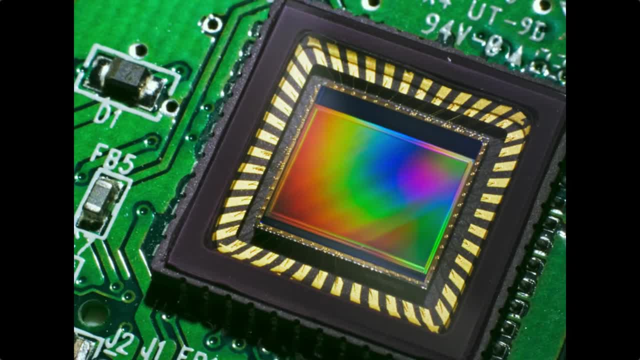 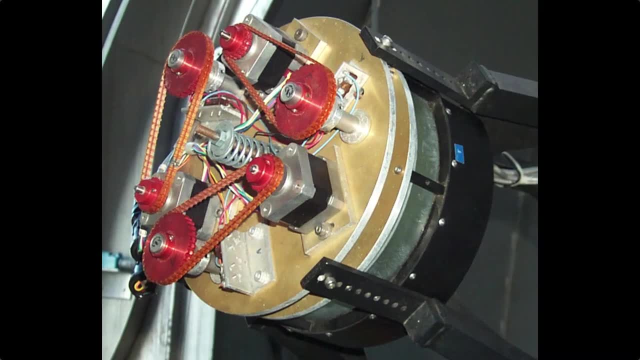 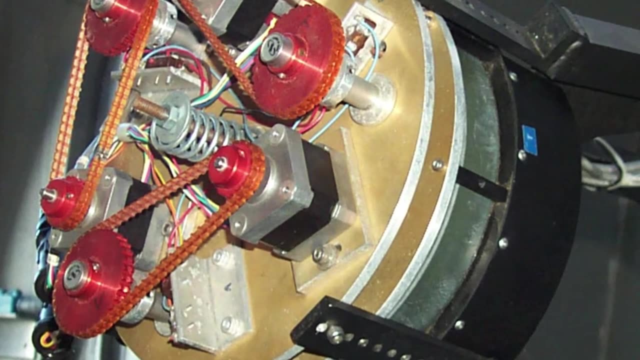 have an electronic charge-coupled device instead of an eyepiece. The telescope is pointed to one small area of the sky. Computer-controlled motors move the telescope to point to exactly the same spot. for many hours, The charge-coupled device continually picks up all sorts of signals. 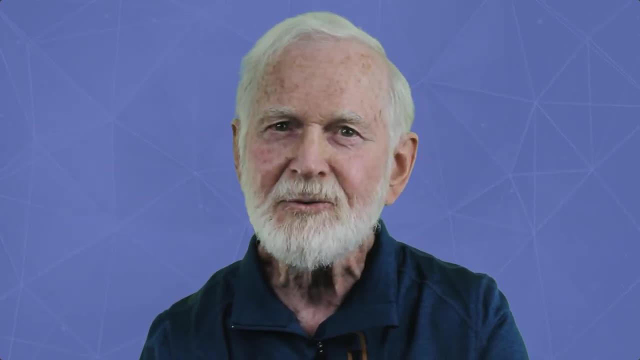 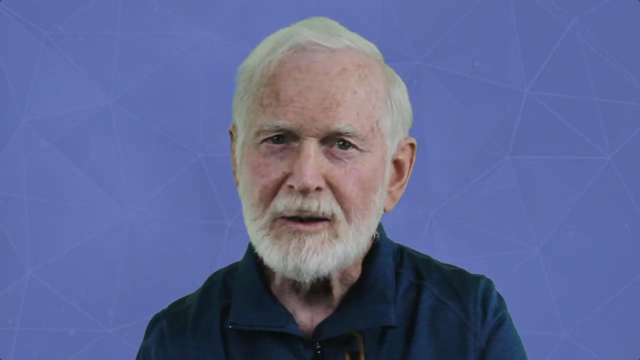 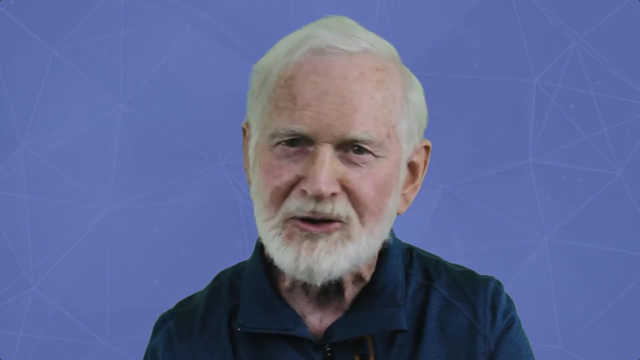 not just light, but infrared, far infrared, ultraviolet x-rays, etc. visible to the human eye. They also pick up normal light far too faint for the eye to see. These signals are fed to a computer all night long. The enormous data files can be handed over. 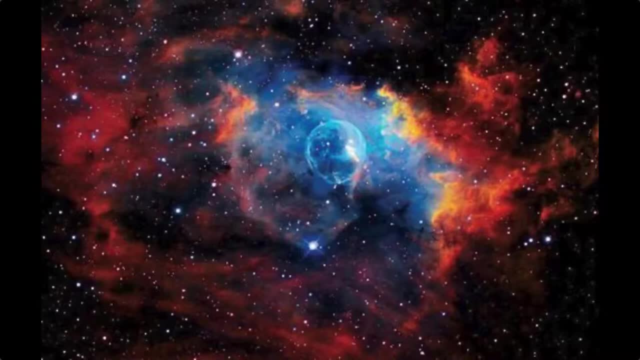 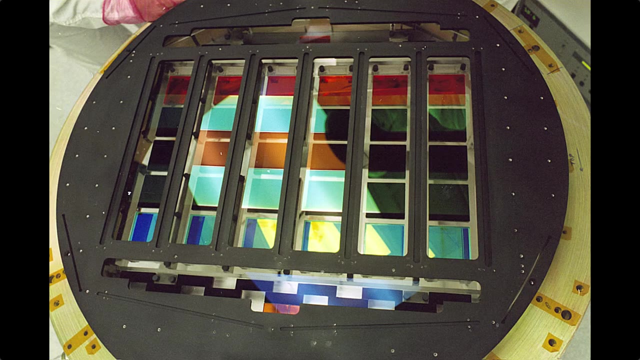 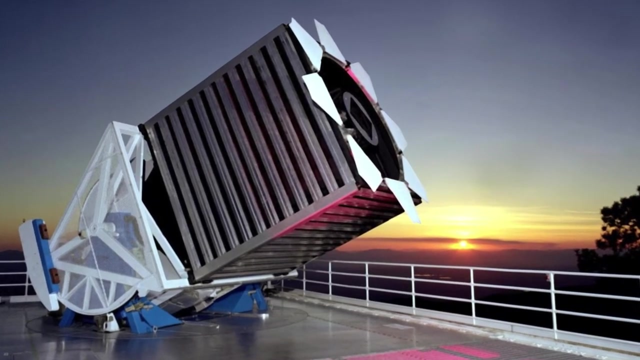 to an astronomer or to an artist to turn into stunning pictures. The largest such charge-coupled camera ever built is being used in the Sloan Digital Skyline. The aim of the Sky Survey is to map galaxies out to the limit of observability. 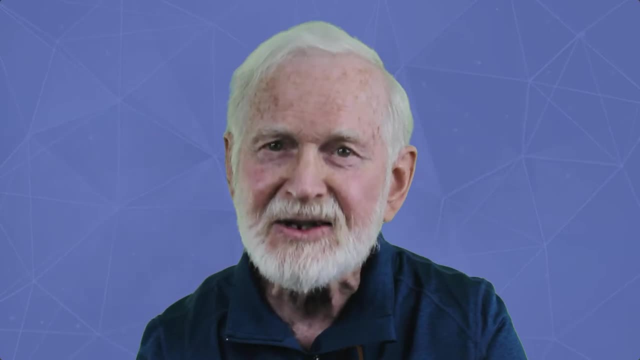 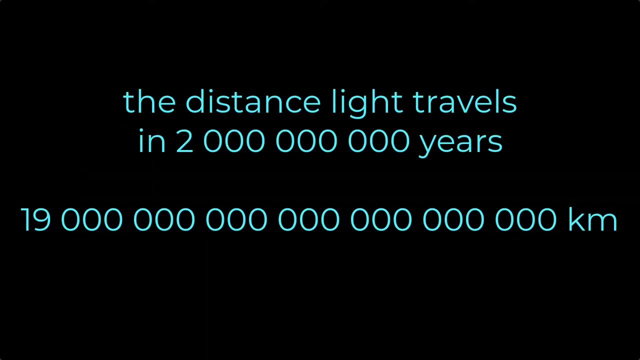 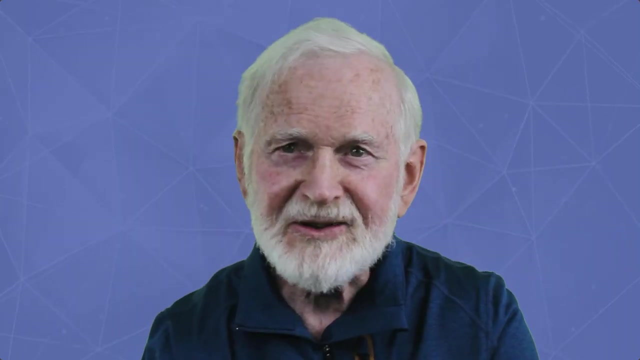 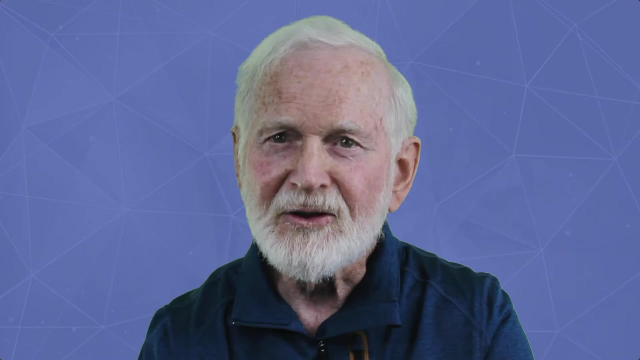 which is said to be 2 billion light-years away, And since light is assumed to travel at 300,000 kilometres a second, that's an astronomically huge number of miles or kilometres away. The project started in 1998.. Pictures were released to the public on the Sloan Sky Survey website in the year 2000,. 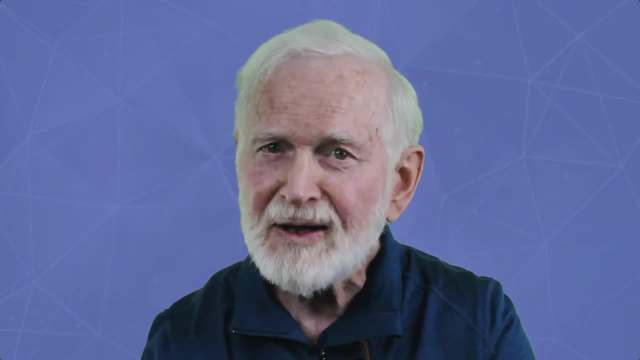 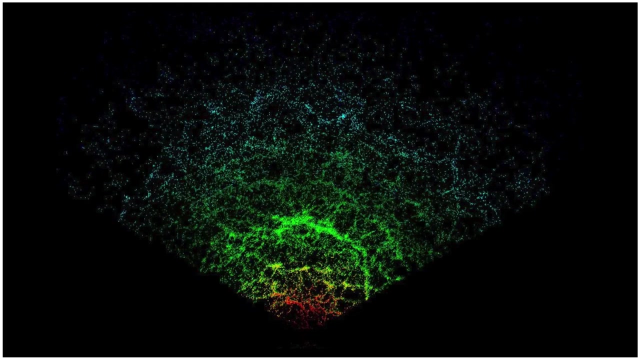 and periodically thereafter, In October and November 2003,. pictures were released which showed a slice of the sky. The astronomers of the world were stunned. The picture shows that we are surrounded by concentric structures where the density of galaxies increases by a fraction of the size of the galaxy. The picture shows that we are surrounded by concentric structures where the density of galaxies increases by a fraction of the size of the galaxy. 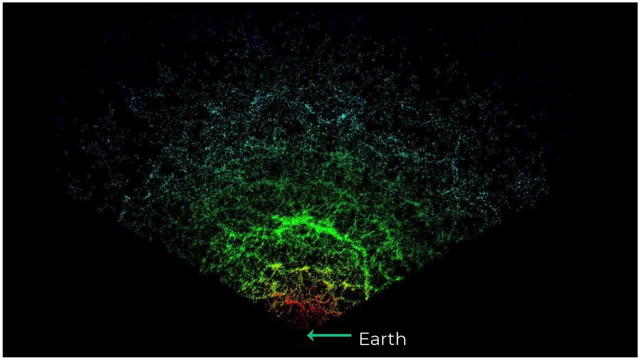 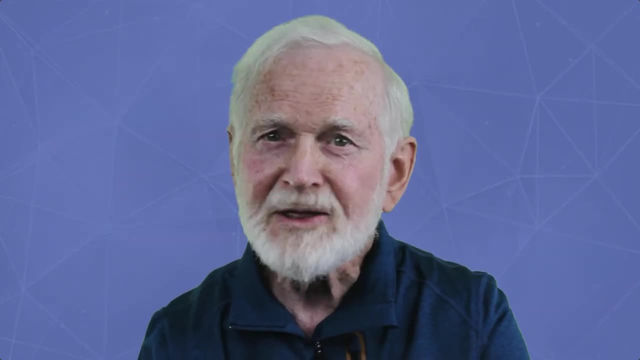 The picture shows that we are surrounded by concentric structures where the density of galaxies increases and decreases periaodically with distance from the Earth. The rings become less dense with increase distance from the Earth. This result was horrifying. There should have been a nearly empty area where the 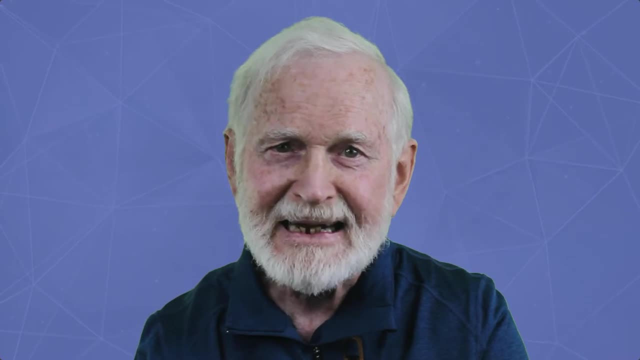 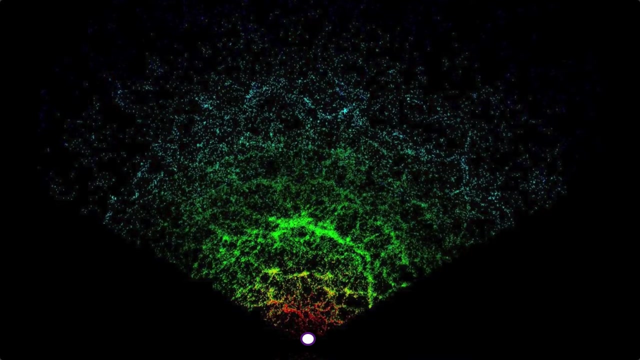 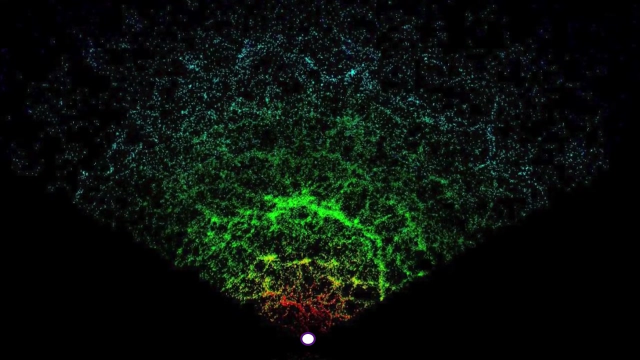 big bang happened surrounded by galaxies getting gradually denser with increasing distance away from the big bang. But the galaxies are concentrated in ballast zust regions, This in bands around the Earth. They become less dense with increasing distance away from the Earth. 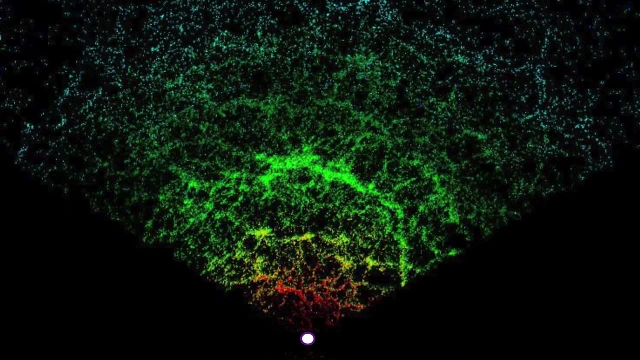 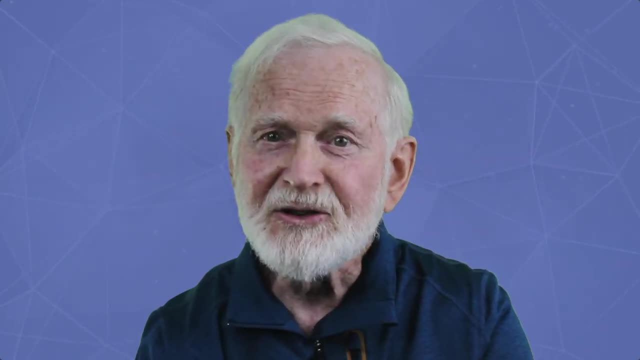 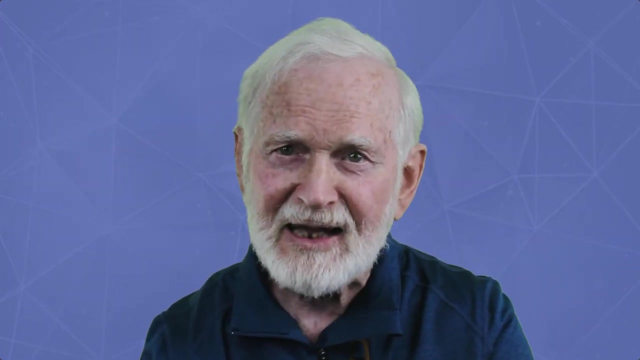 The Earth is at the centre of the universe and it was supposed to be nowhere special. In the most recent data release, release 17,, there's a new map with two slices. The upper slice is a revised version of the one from 2003.. 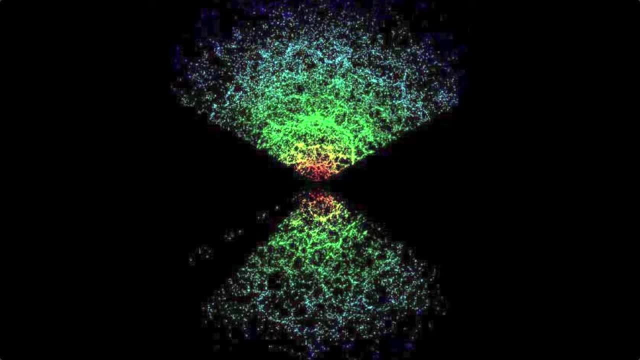 Many more galaxies have been added. The new lower slice has far fewer galaxies, but presumably more will be added as observations continue. The rings around the Earth are not as clear as in the upper slice, but when more data gets added, I expect they'll show up just as clearly. 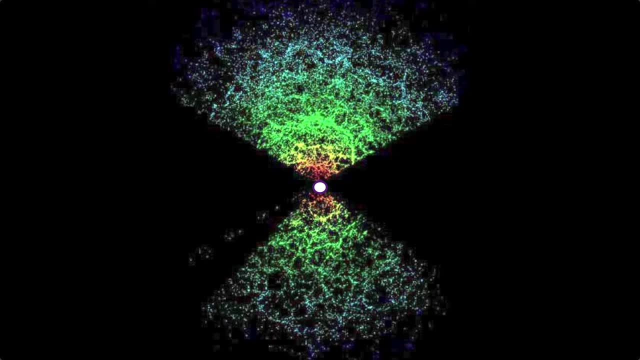 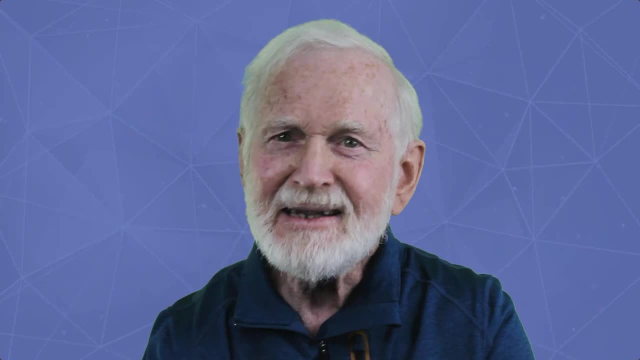 Both slices show that the Earth is at the centre of everything, But astronomers don't only use optical telescopes. In 1967, Arnaud Penzias and Robert Wilson surprised the world. They'd pointed their microwave detector at the sky and found, to their amazement- 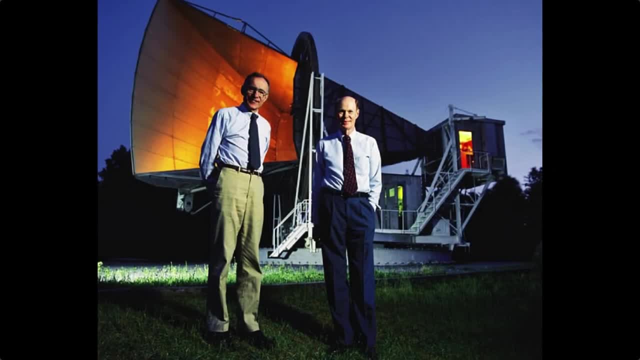 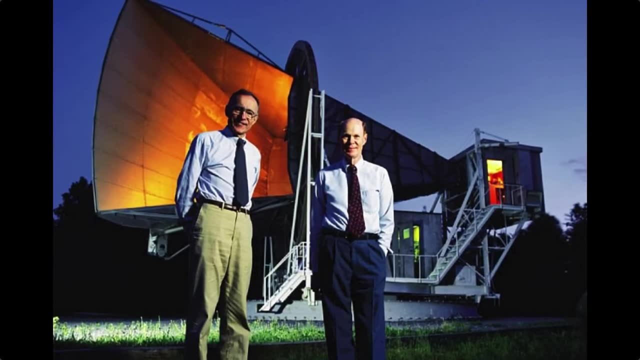 that wherever they pointed it, they got a constant signal close to minus 270 degrees Celsius, about 4 degrees absolute. This means that the Earth is at the centre of the universe, But astronomers don't only use optical telescopes. In 1967, Arnaud Penzias and Robert Wilson. 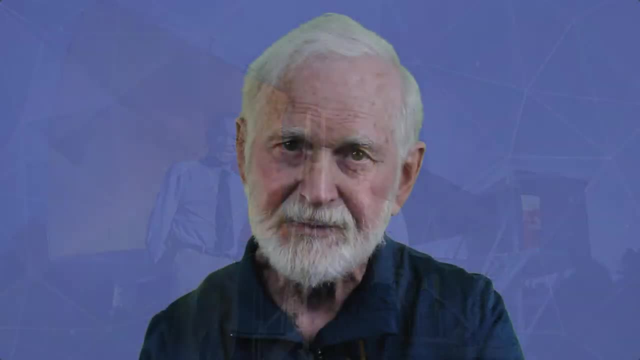 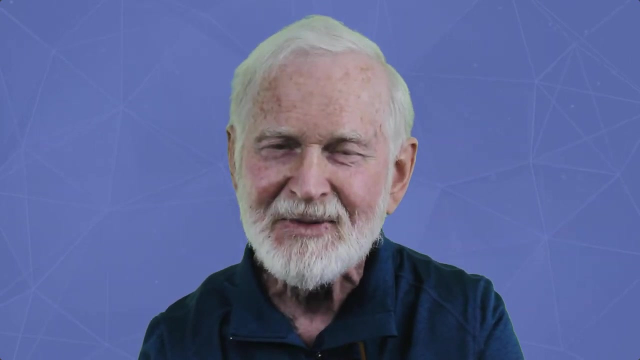 surprised the world. They'd pointed their microwave detector at the sky. some Big Bang experts clapped their hands and said: oh, this must be the echo of the Big Bang. So Penzias and Wilson got a Nobel Prize for proving that the Big Bang 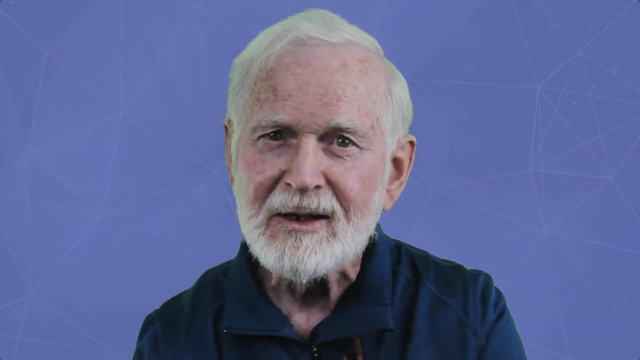 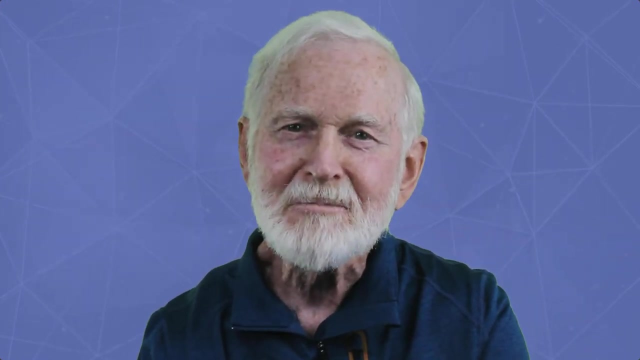 was not just speculation, but something with an observable echo, but something with an observable echo. The echo was soon given the name cosmic background radiation and a diagram was devised to represent it. and a diagram was devised to represent it. and a diagram was devised to represent it. 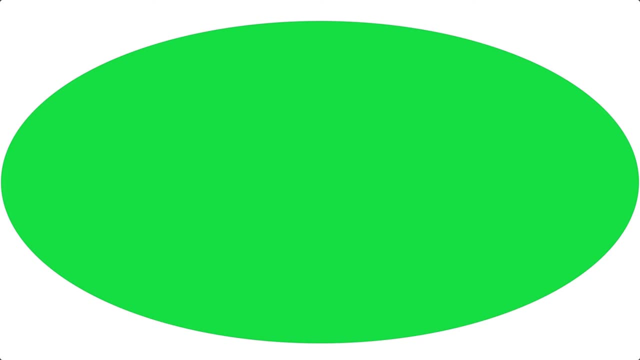 It's a bit tricky to visualise because the diagram represents a sphere all around you As you look at the top of the ellipse. As you look at the top of the ellipse, that's directly overhead, The bottom of the ellipse is directly below you. 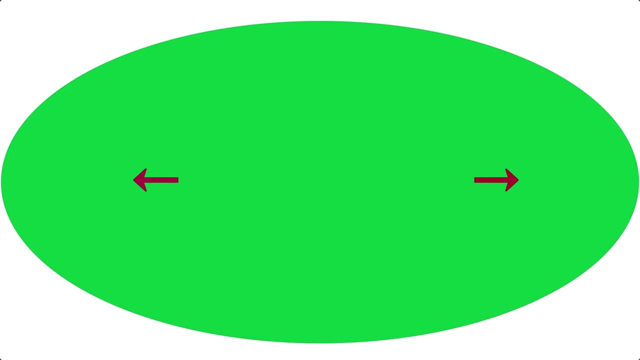 and the narrow sides of the ellipse are behind you. Both thin ends of the ellipse are at the same point, directly behind the middle of your back. The long axis is in the direction of the ellipse's ecliptic, the plane in which the heavenly bodies 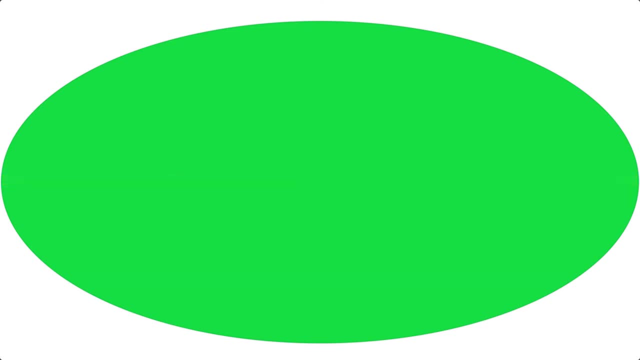 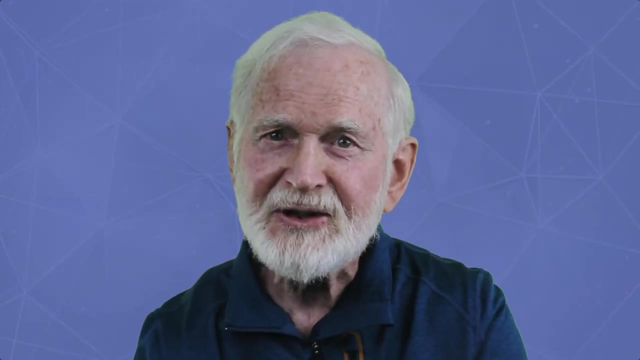 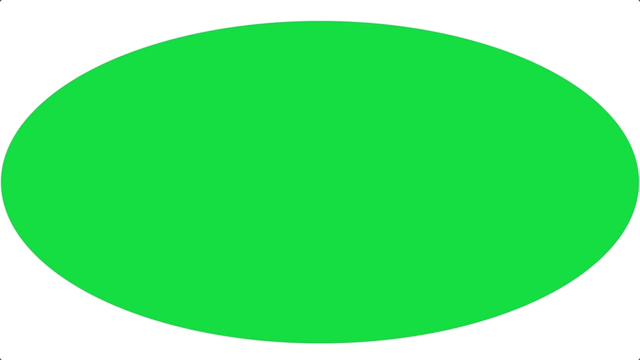 orbit the Earth, By far the most convenient reference line for an astronomer. But there was a problem. To the best accuracy, anybody could measure to anybody could measure to, it was perfectly uniform. But if this was an echo of the Big Bang? 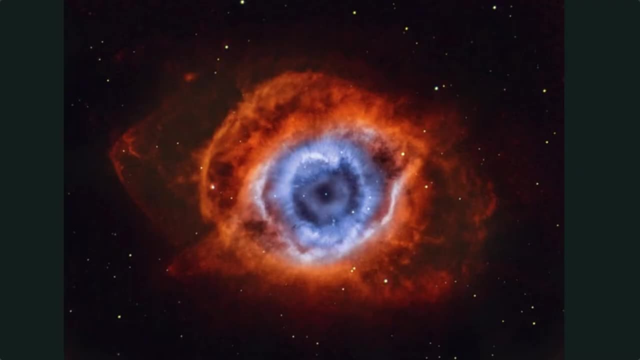 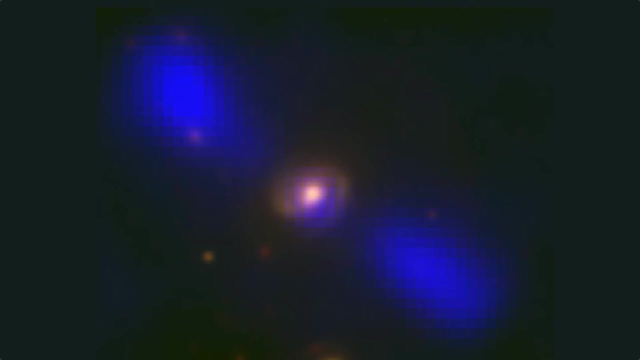 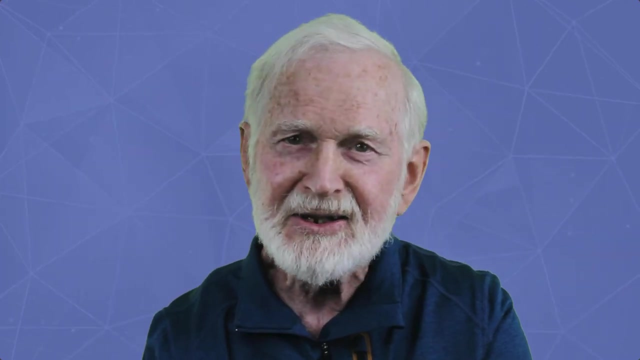 it should have been lumpy, Since the Big Bang is lumpy with huge galaxies and clusters of galaxies here and huge empty spaces there. The Big Bang theory was changed to try and make it smoother. Brilliant ideas were tried, like having the first. 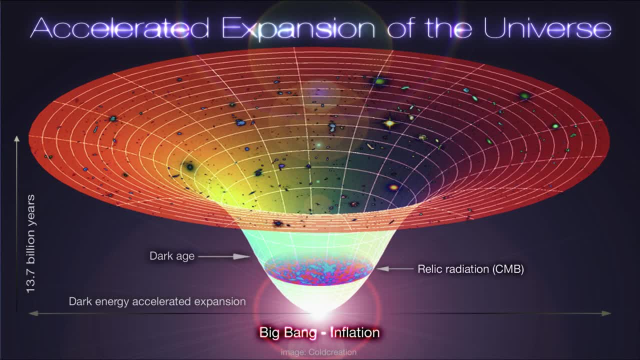 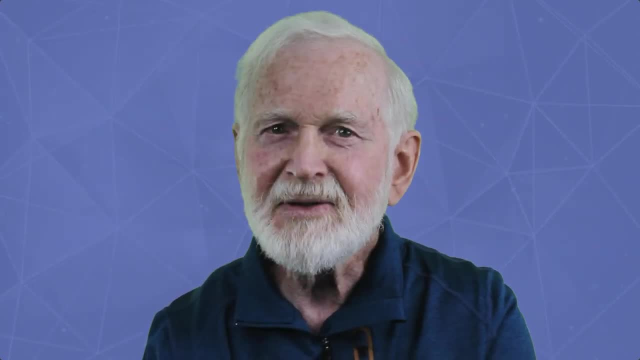 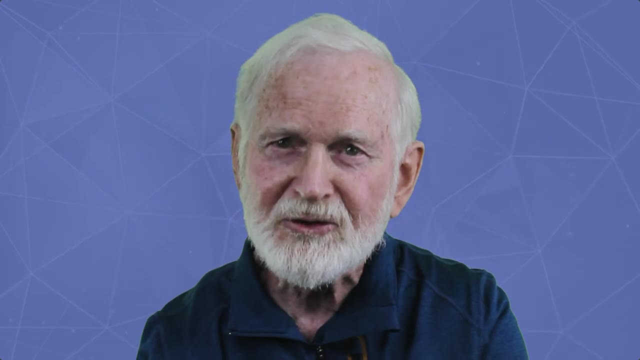 milli-microsecond inflating, expanding at millions of times faster than the speed of light and suddenly slowing down again. But even that couldn't make the Big Bang anywhere near smooth enough. So the astronomers launched ultra-sensitive instruments into space to measure. 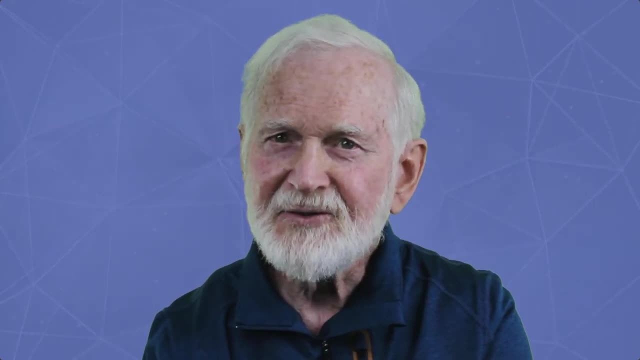 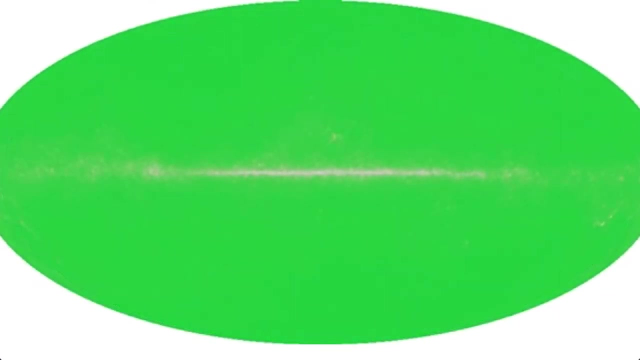 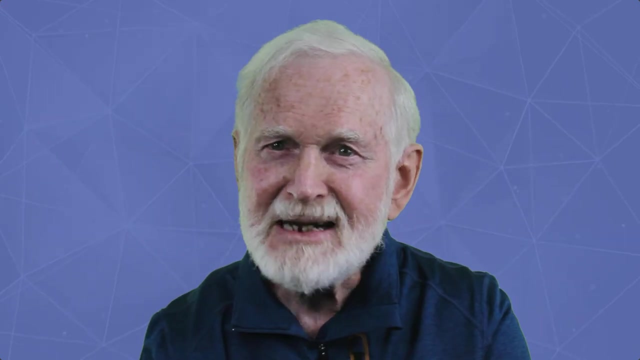 to ten-thousandths of a degree. They finally got such sensitive instruments. they could detect a pattern in the measurements. But, horror of horrors, it was an axis, An axis corresponding with the Earth's ecliptic. It was immediately named the axis of evil. 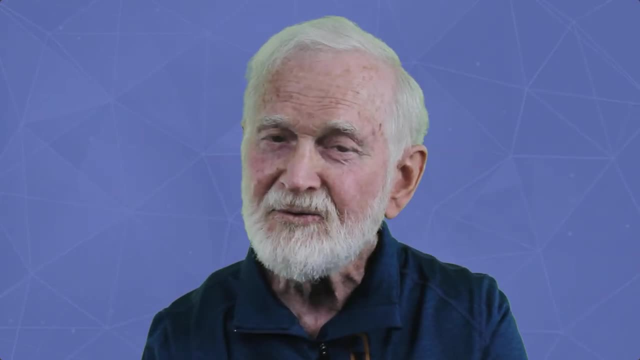 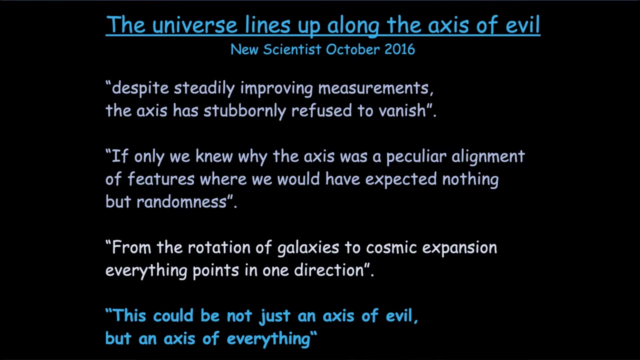 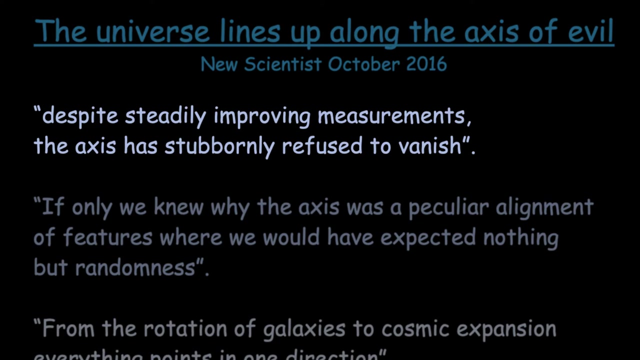 It must be very evil. It pointed to the Earth as something special, And the more they looked, the more they found to despair about. as Clarke pointed out in The New Scientist, Despite steadily improving measurements, the axis has stubbornly refused to vanish. 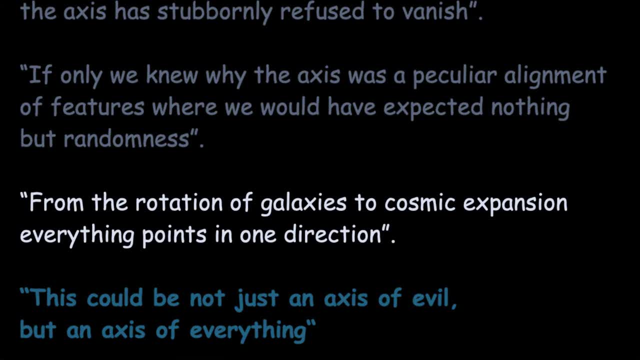 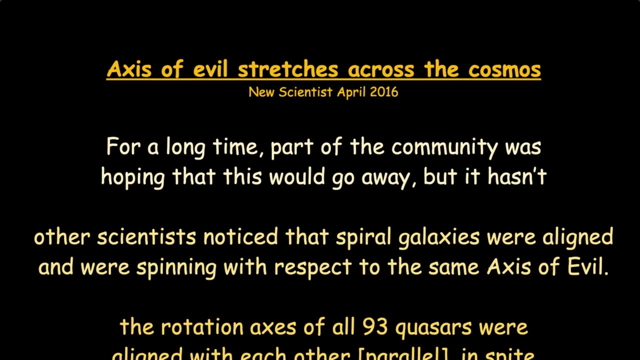 From the rotation of galaxies to cosmic expansion, everything points in one direction. This could not only be an axis of evil, but everything. Brooks pointed out that for a long time, part of the community was hoping that this would go away, But it hasn't. 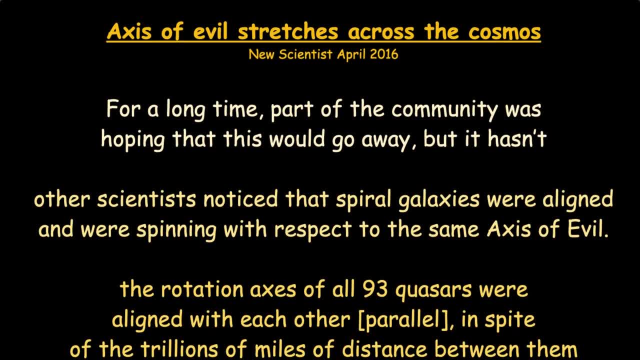 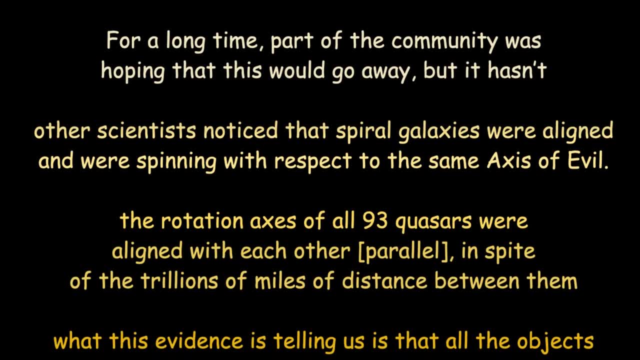 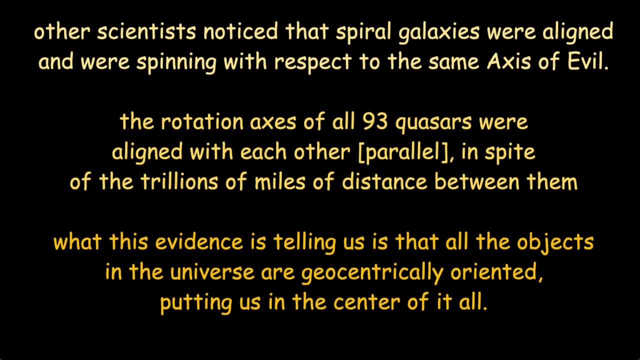 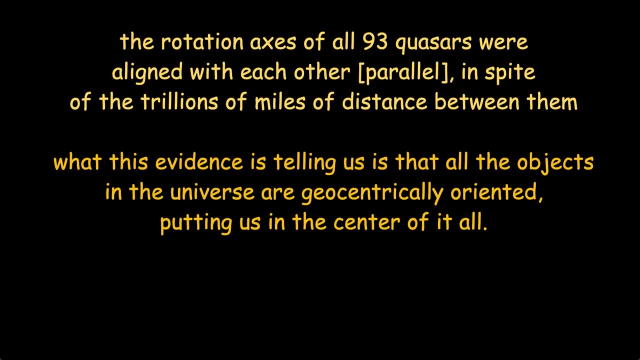 Instead, it was found that other astronomical phenomena were also pointing the same way. Other scientists noticed that spiral galaxies were aligned and were spinning with respect to the same axis of evil, In spite of the trillions of miles of distance between them. What this evidence is telling us? 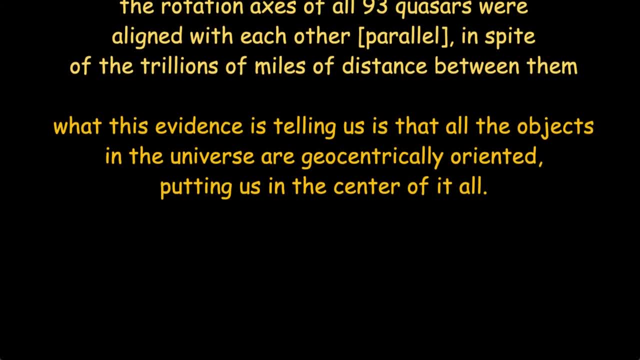 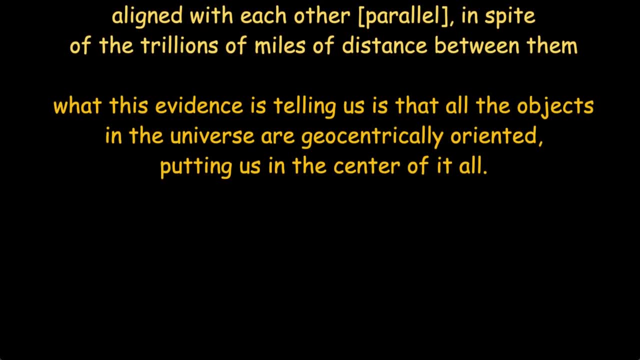 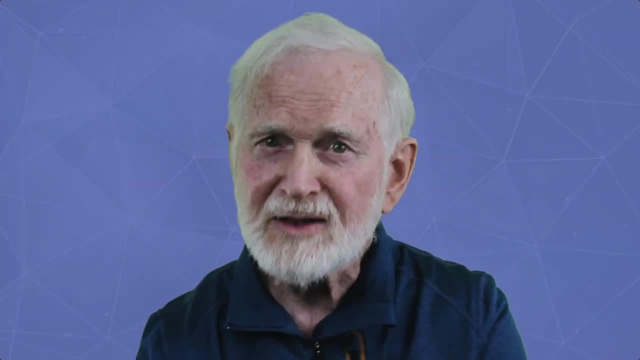 is that all the objects in the universe are geocentrically orientated, putting us in the centre of it. all The three latest papers I can find on it- published in 2020, all conclude that the Big Bang must have been aligned in some way.